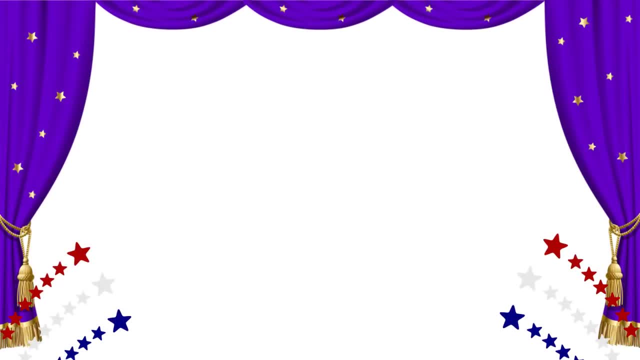 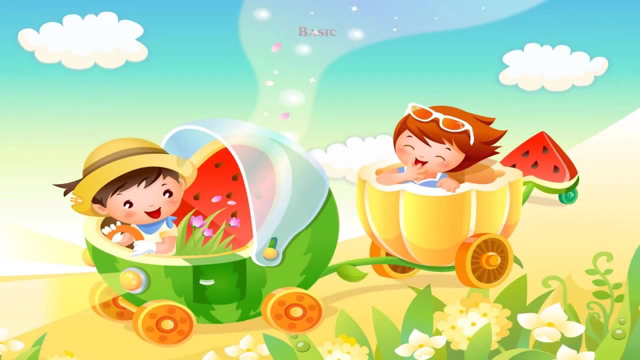 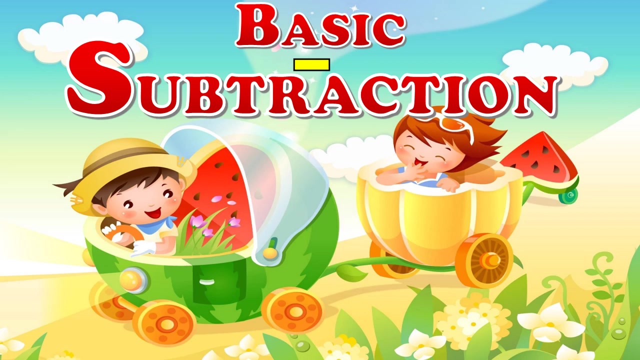 Hello kids, today we will learn about basic subtraction. Subtraction is the process of removing a particular number of objects from given total number of objects. Subtraction could be said as finding the difference between numbers, ie taking one number from another, and this subtraction is denoted by sin-. Now let's get to know. 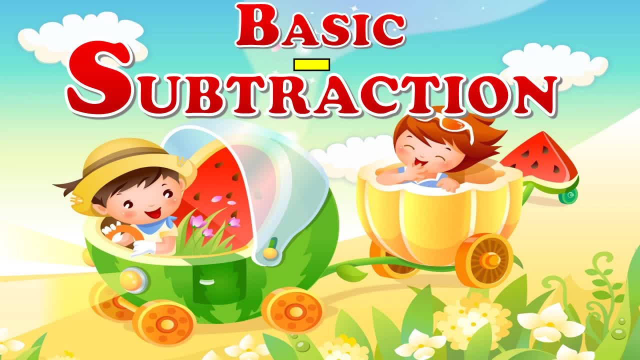 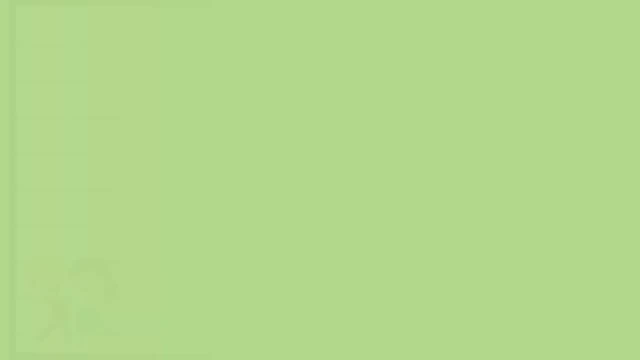 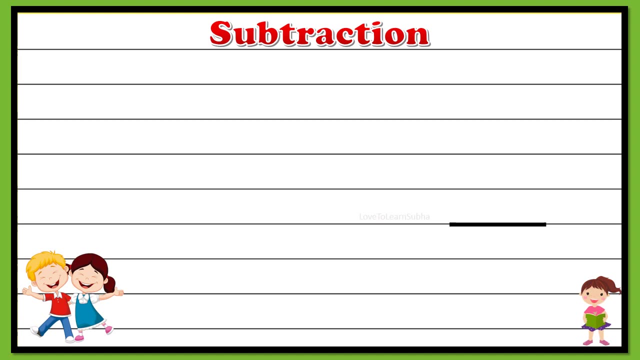 about this basic subtraction process, with few examples, along with the pictures. Now let's get started. Now let's understand the process of subtraction with this example. Now let's check out what are the objects available. So here we have one, two, three. So totally we have three. 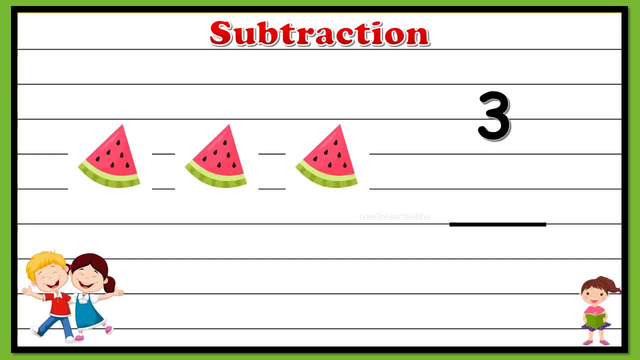 pieces of watermelon, Since we have two kids, so each one would have taken one piece each. So we have to minus two. Now let's check out the remaining balance. So when we do minus one, two, So the remaining piece of watermelon is one. So three minus two gives us one. So 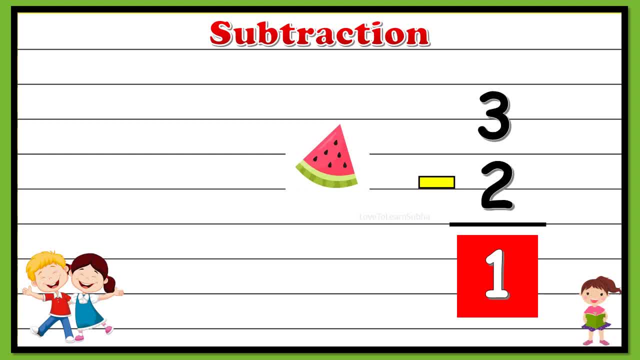 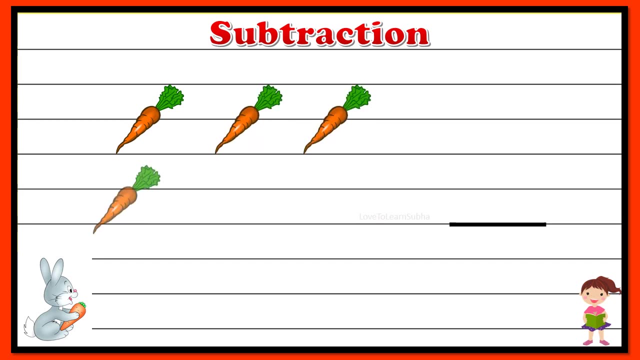 one is the difference between three minus two. Now let us take another example to understand this subtraction. So here we have 1,2,3,4,5,6, So totally we have 6 carats. So in this the bunny takes 4 of the carats, So we put it as minus 4.. 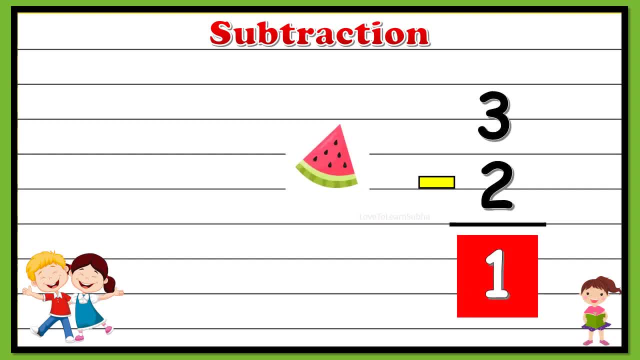 one is the difference between three minus two. So three minus two is equal to one. So in this case we have one. Now let's look at too, Now let us take another example to understand this subtraction. So here we have 1,, 2,, 3,. 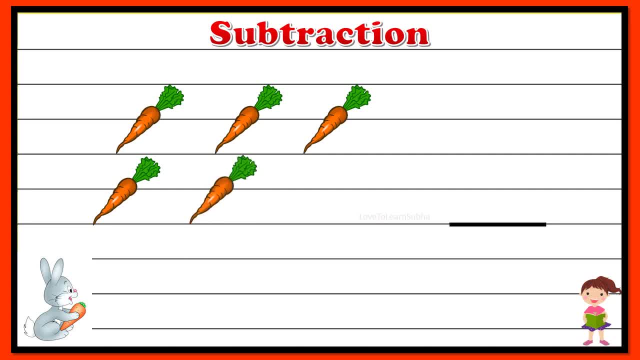 4, 5, 6.. So totally we have 6 carats. So in this the bunny takes 4 of the carats, So we put it as minus 4.. Now let us see how this subtraction works and what is the remaining. 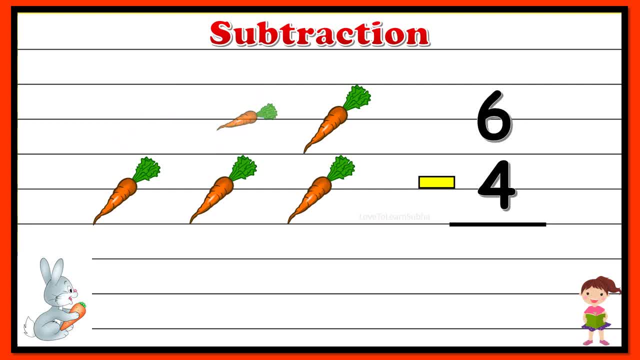 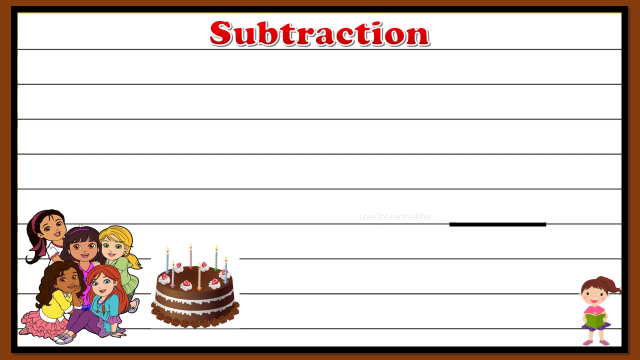 balance: 1, 2, 3, 4.. So we are subtracting 4 from 6.. So the balance is 1, 2.. So we have 2 carats left out. So 6 minus 4 gives you 2.. Now let us check out another example Here: Dora and her. 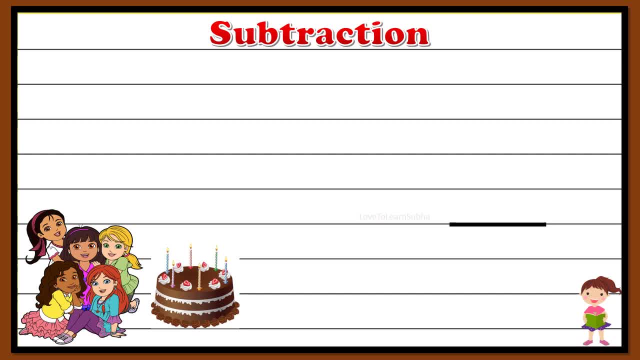 friends are on the birthday party. So here let us check out what is the object available: 1,, 2,, 3,,4,,5,,6,,7,,8.. So totally there are 8 pieces of cake And since there are 5 friends, so we have to minus. 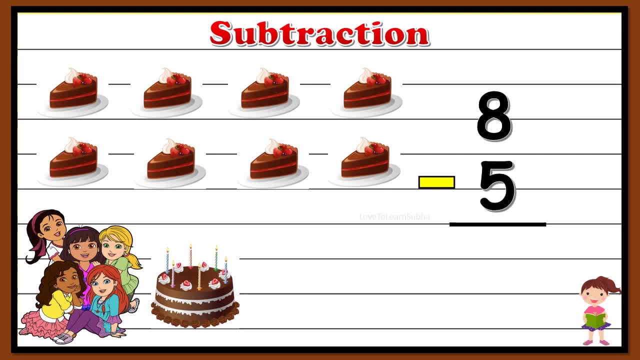 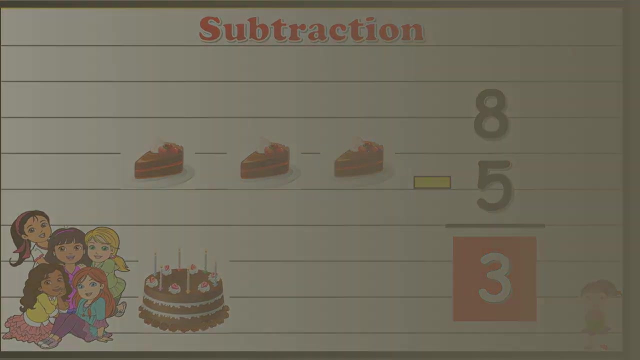 5 pieces of cake. pieces of cake. now let's check out the remaining balance. so to find the remaining balance, let's start counting 1, 2, 3, 4, 5. so after subtracting 5, let's see the balance: 1, 2, 3. so 8 minus 5 gives you the value 3. now let's understand the 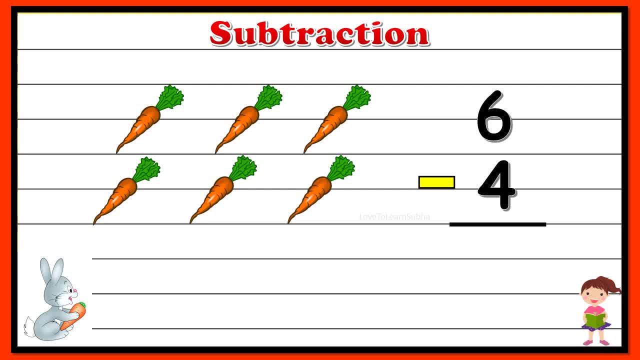 Now let us see how this subtraction works and what is the remaining balance: 1,2,3,4. So we are subtracting. So we are subtracting 4 from 6. So the balance is 1,2.. So we have 2 carats left out. So 6 minus 4 gives you 2.. 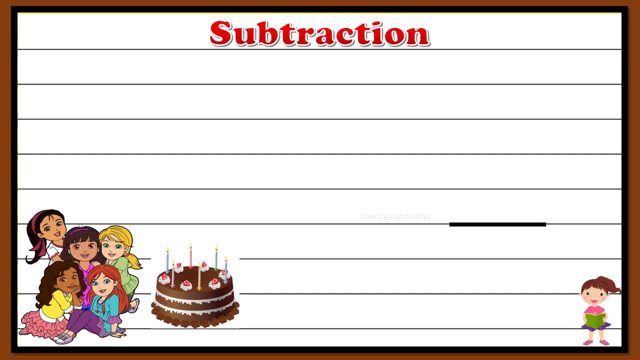 Now let us check out another example. Here, Dora and her friends are on the birthday party, So here let us check out what is the object available: 1,2,3,4,5,6, 2,3,4,5,6,7,8. 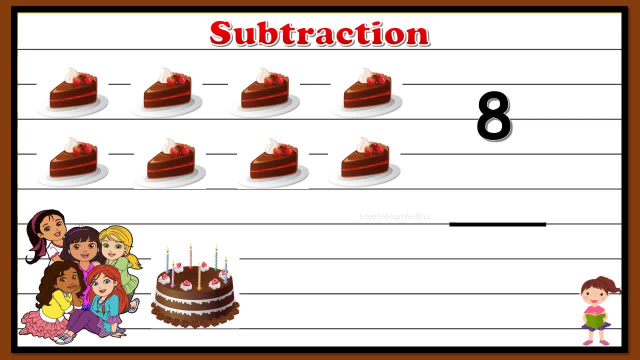 So, totally, there are 8 pieces of cake And since there are 5 friends, so we have to minus 5 pieces of cake. Now let us check out the remaining balance. So in the remaining balance, let us start counting 1,2,3,4,5. 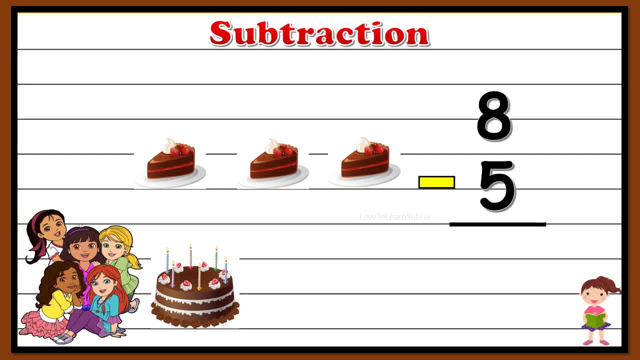 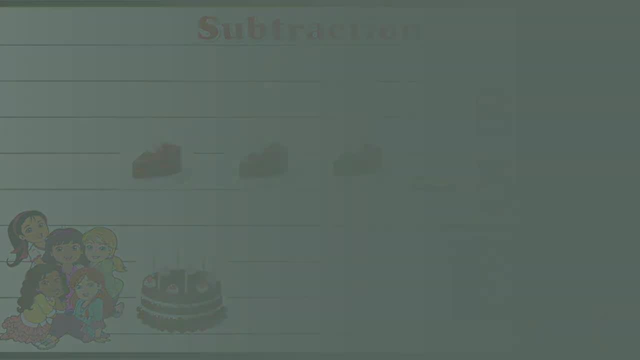 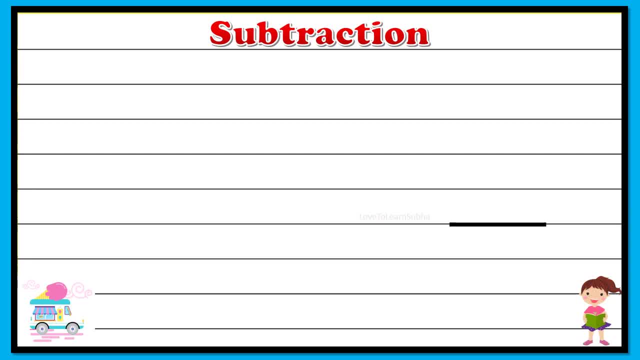 So 8 minus 5 gives you the value 3.. Now let us understand the concept of subtraction with another example here: Here we have an ice cream cart. Now let us see how many ice cream cones are available. Here we have an ice cream cart. Now let us see how many ice cream cones are available. 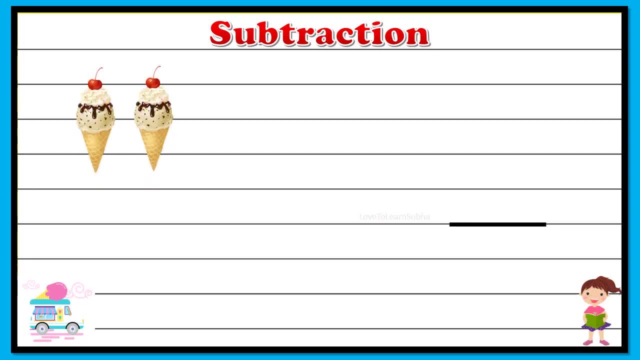 Here we have an ice cream cart. Now let us see how many ice cream cones are available: 1,2,3,4,5,6,7,8 and 9.. So there are totally 9 pieces of ice cream available. 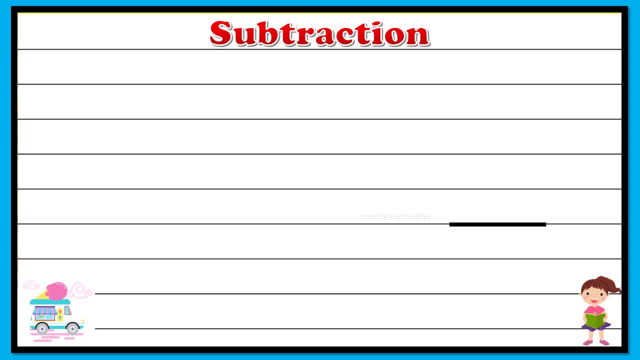 concept of subtraction with another example here. here we have an ice cream cart. now let's see how many ice cream cones are available. you 1, 2, 3, 4, 5, 6, 7, 8 and 9, so there are totally 9 pieces of ice cream available. 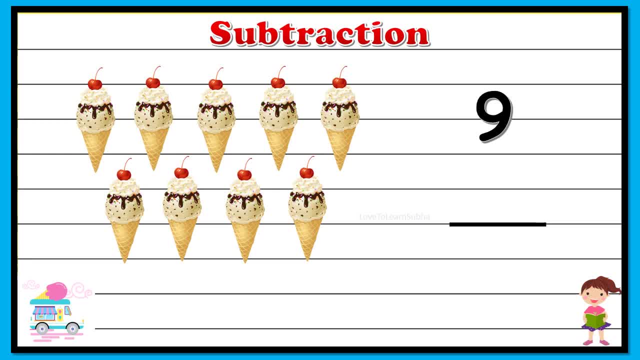 now let's assume that in that ice cream we have 4 pieces got sold out, so we have to write it as minus 4. now we have to find what is the balance left out. now let's start counting to find the remaining balance: 1, 2, 3, 4. so now we have. 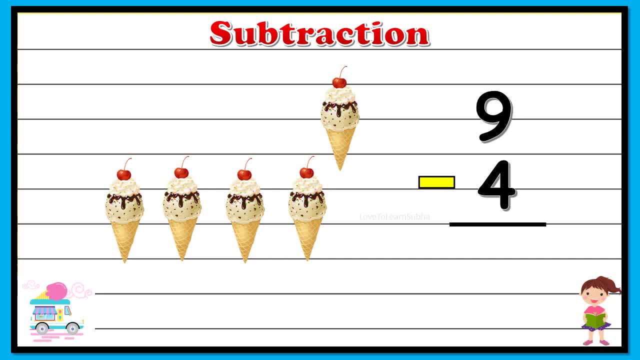 subtracted 4 ice creams from total 9 ice creams, flight 9 to place balance. now let's check out the remaining balance. so we have 1, 2, 3, 4, 5. so totally get a 5 ice creams remaining. so 9 minus 4 gives you. 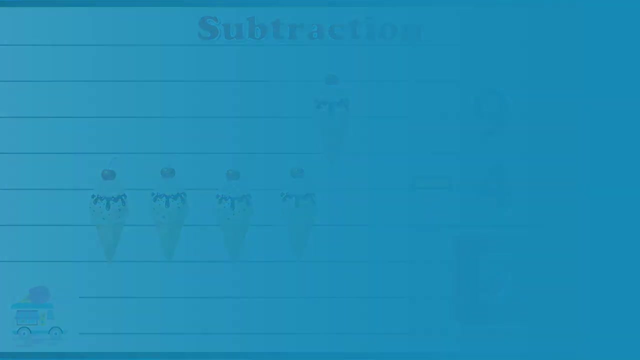 the value 5. now let's check out another example: 1, 2, 3, 4, dis数 5, kiss 5, guess 263, especially. let's check out that remaining balance. so we have 1, 2, 3, 4, 5, so totally there are 5 ice creams remaining. so 9 minus 4 gives you the value 5. now let's check out another example. 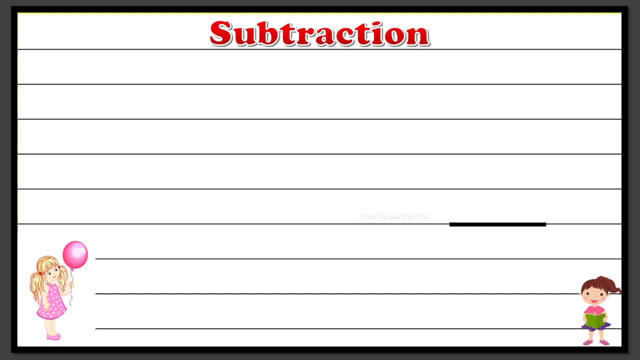 sample to understand this subtraction. Now let's find out what is the object available here. So we have 1, 2, 3, 4,, 5, 6,, 7,, 8,, 9,, 10.. So totally we have 10 balloons available. 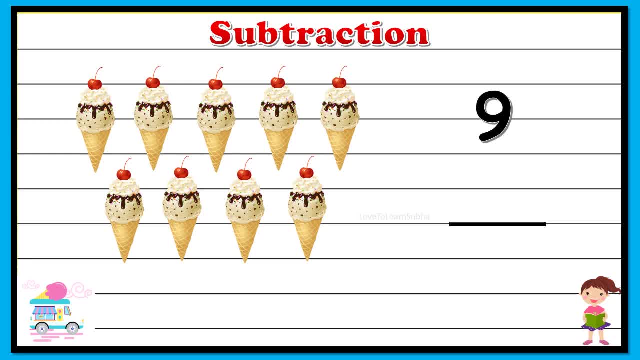 Now let us assume that in that ice cream we have 4 pieces got solid. Now let us assume that in that ice cream we have 4 pieces got solid out, So we have to write it as minus 4.. Now we have to find what is the balance left out. 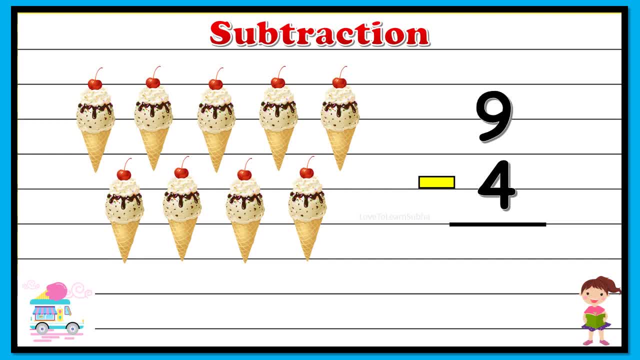 Now let's start counting to find the remaining balance: 1,, 2,, 3,, 4.. So now we have subtracted 4 ice creams from total 9 ice creams. Now let's check out the remaining balance. So we have 1,, 2,, 3,, 4, 5.. So totally there are 5 ice creams remaining. So 9 minus 4 gives 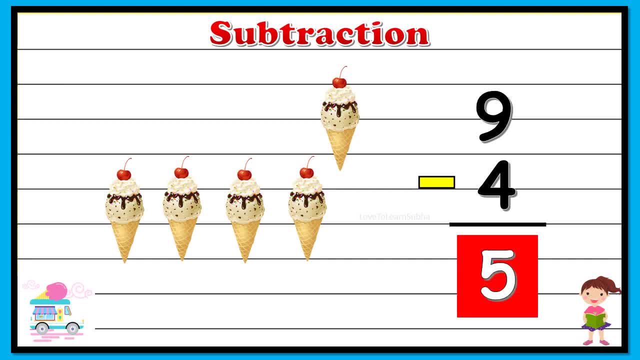 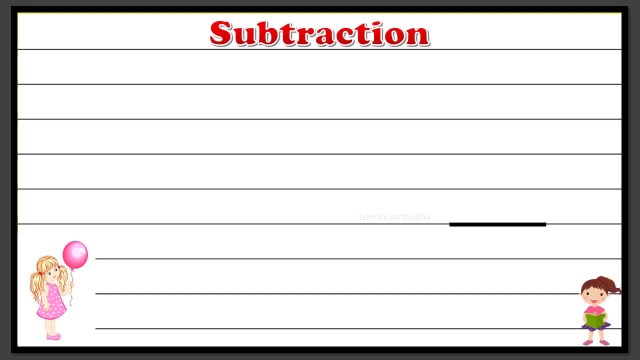 you the value 5.. Now let's check out another example to understand this subtraction. Now let's find out what is the object available here. So we have 1,, 2,, 3,, 4,, 5,, 6,, 7,, 8,, 9,, 10.. So totally there. 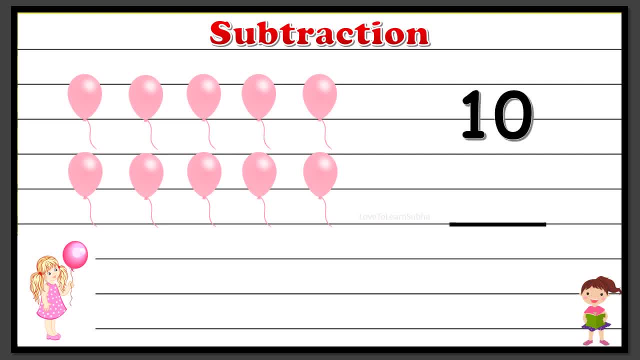 are 5 ice creams available here. Now let's check out another example to understand this subtraction. So we have 1, 2,, 3, 4,, 5, 6,, 7,, 8,, 9, 10.. So, totally, there are 5 ice creams available here. 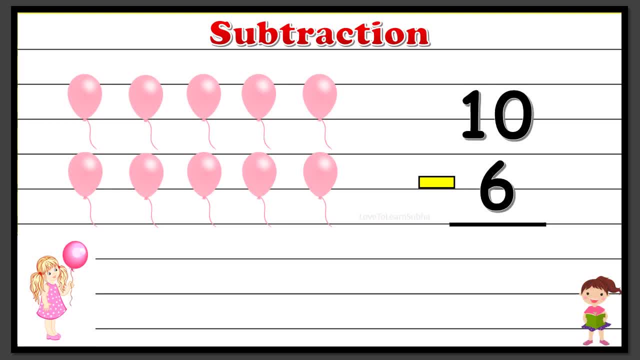 So we have 1,, 2,, 3,, 4,, 5,, 6,, 7,, 8,, 9,, 10.. So, totally, there are 5 ice creams available here. So here, 6 balloons got flew away. So here, 6 balloons got flew away. Now let's start counting. 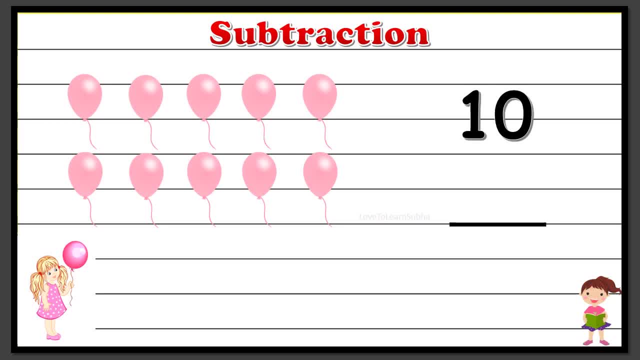 here, In that let us assume that 6 of the balloons flew away, So we take it as minus 6.. Now let's start counting the objects to find the remaining balance. So we have to subtract 6.. 1,, 2,, 3,, 4,, 5,, 6,, 7,, 8,, 9,, 10.. So we have 1,, 2,, 3,, 4,, 5,, 6,, 7,, 8,, 9,, 10.. So totally we have 1,, 2,, 3,, 4,, 5,, 6,, 7,, 8,, 10.. So totally, we have 1,, 2,, 3,, 4,, 5,, 6,, 7,. 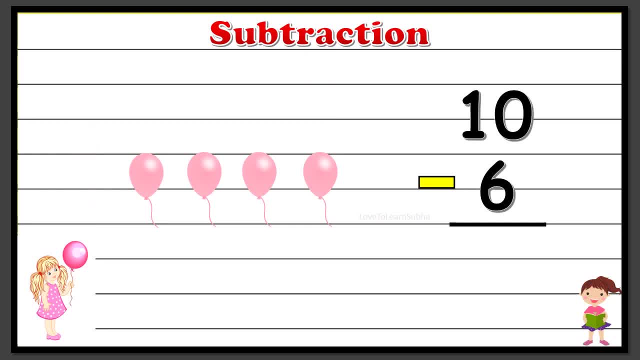 10.. So totally, we have 1,, 2,, 3,, 4,, 5,, 6,, 7,, 8,, 10.. So here, 6 balloons got flew away. Now let's start counting the balanced balloons. We have 1., 2., 3., 4.. So balanced, we have 4. 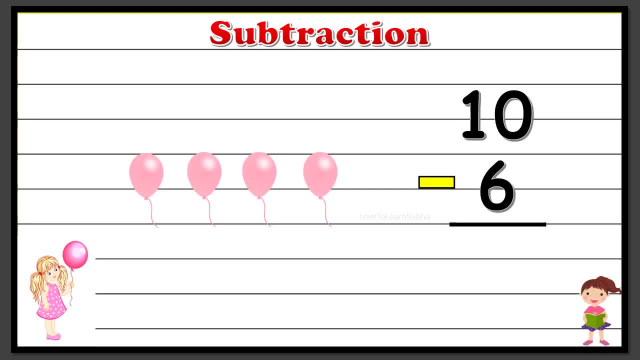 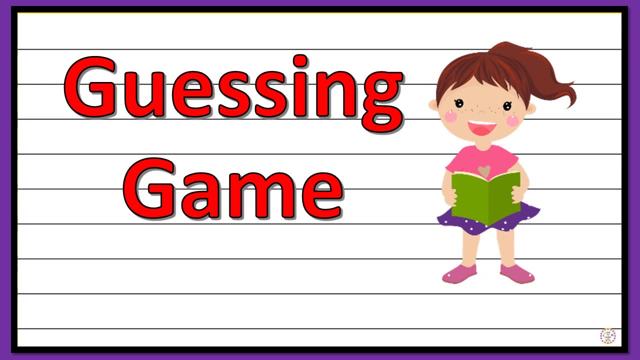 balloons left out. So 10 minus 6 gives you the value 4.. Now let's play a game. We will play a guessing game Here. I'll be giving you some set of pictures and you have to find the difference. So I'll be giving you the total number of pictures and in that you have 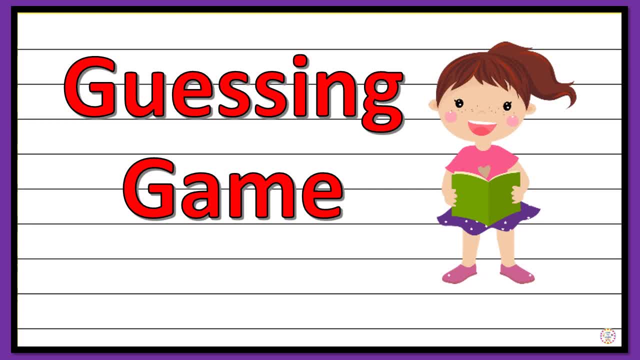 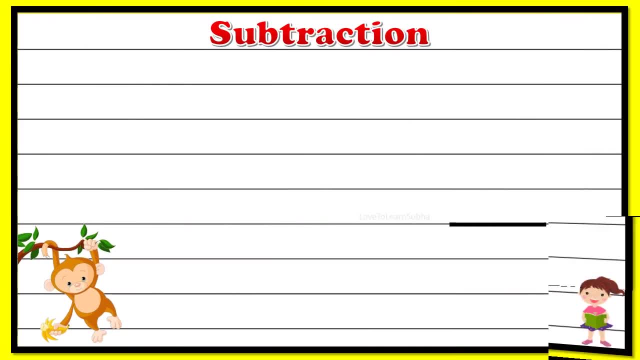 to subtract a particular number of pictures and find the remaining balance. So now let's get started. So here is our first example problem. Now let's check out what is the object available? 1, 2,, 3, 4, 5.. So totally, we have 5 bananas. Now let's assume that from 5, 3 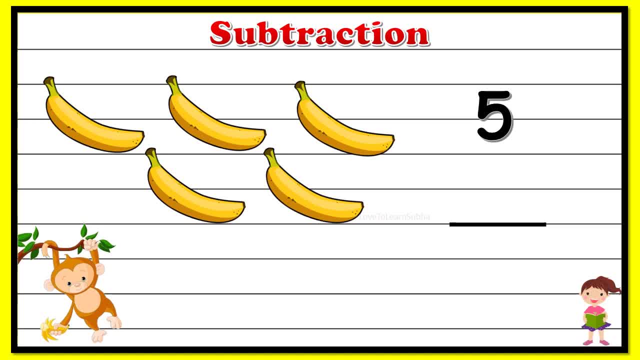 bananas are taken away by this monkey, So we write it as minus 3.. Now you have to find the balance bananas. Now let's check out the remaining balance, and for this we have to start counting the objects 1,, 2,, 3.. So from 5 bananas we have subtracted 3 bananas. Now let's count the. 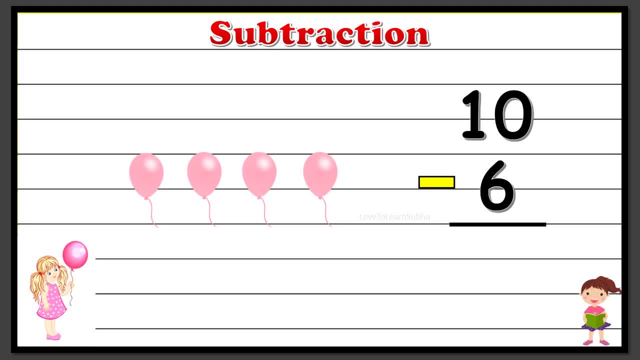 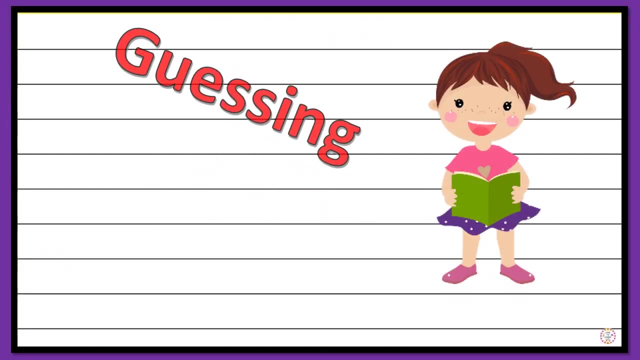 the balance: balloons 1… 2… 3… 4.. So balance: we have 4 balloons left out. So 10 minus 6 gives you the value 4. 4 better. Now let's play a guessing game Here. I'll be giving you some set of pictures and you 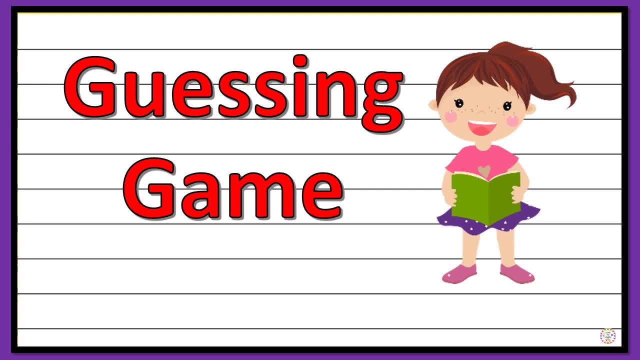 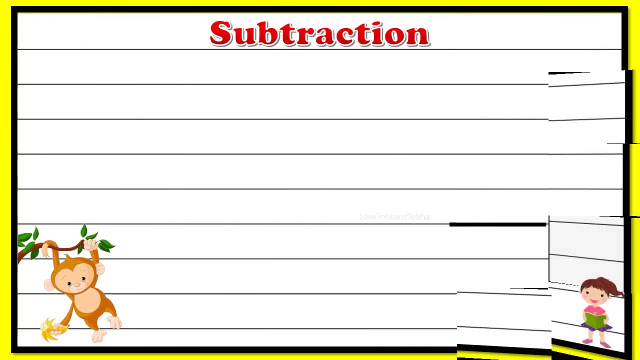 have to find the difference. So I'll be giving you the total number of pictures and in that you have to subtract a particular number of pictures and find the remaining balance. So now let's get started. So here is our first example problem. Now let's check out what. 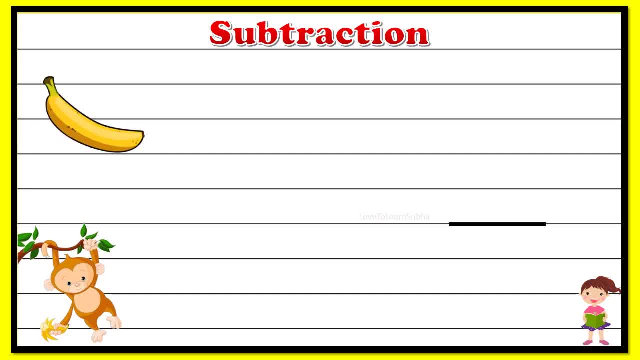 is the object available 1, 2,, 3,, 4, 5.. So, totally, we have 5 bananas. Now let's assume that from 5, 3 bananas are available. So let's assume that from 5, 3 bananas are available. 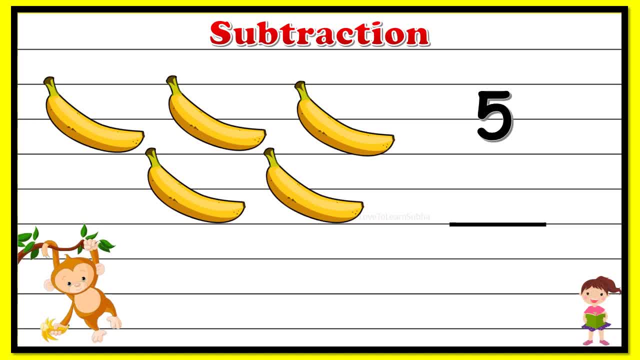 So from 5,, 3 bananas are taken away by this monkey, So we write it as minus 3.. Now you have to find the balance bananas. Now let's check out the remaining balance, and for this we have to start counting the objects. 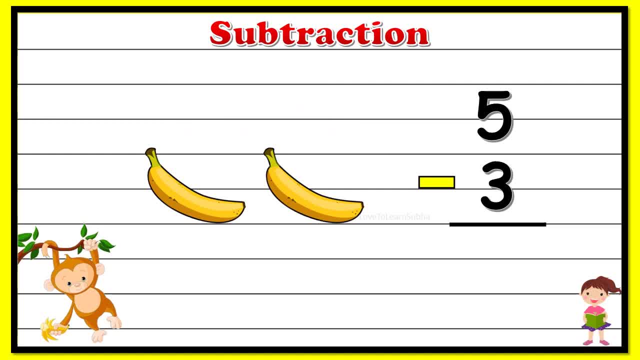 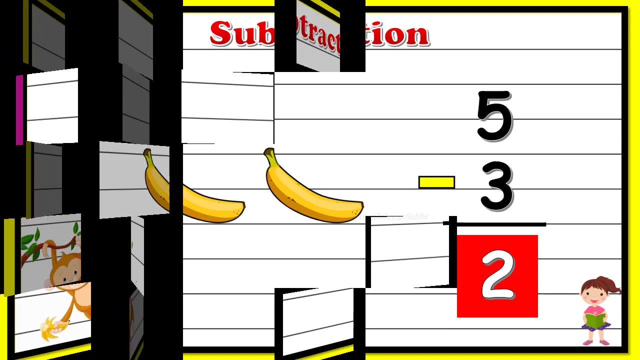 1, 2, 3.. So from 5 bananas we have subtracted 3 bananas. Now let's count the remaining 1, 2.. So 5 minus 3 gives you the value 2.. So we have 2 bananas remaining. Now let's. 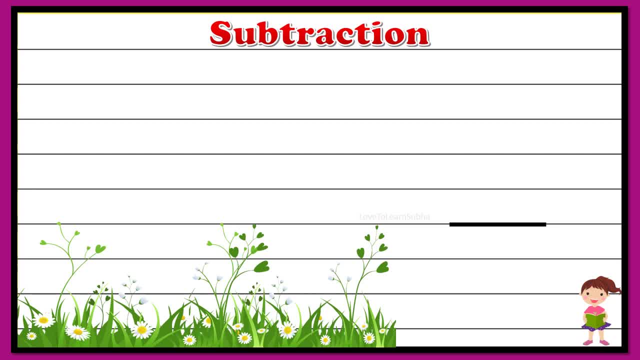 take another example problem here. Now let's see what is the object available. We have 1,, 2,, 3,, 4,, 5,, 6,, 7.. So totally we have 7 butterflies. Now let's assume that from 7, the 4 butterflies got flew away. So